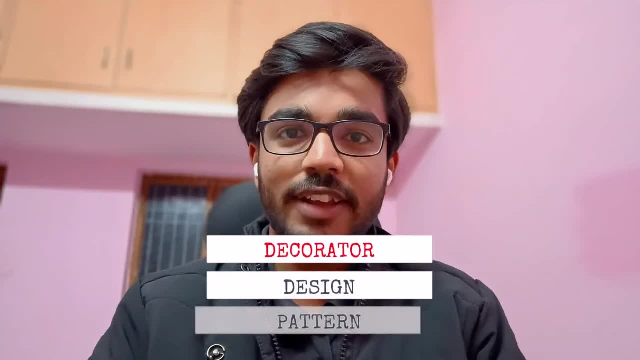 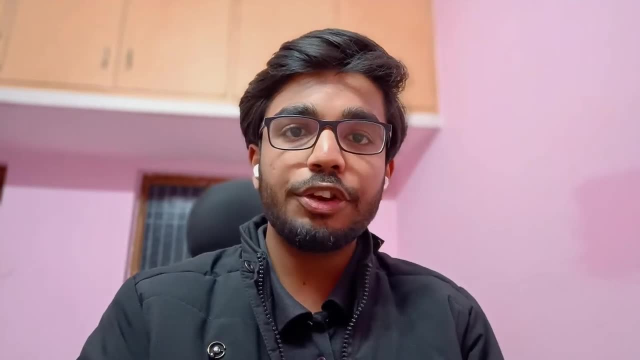 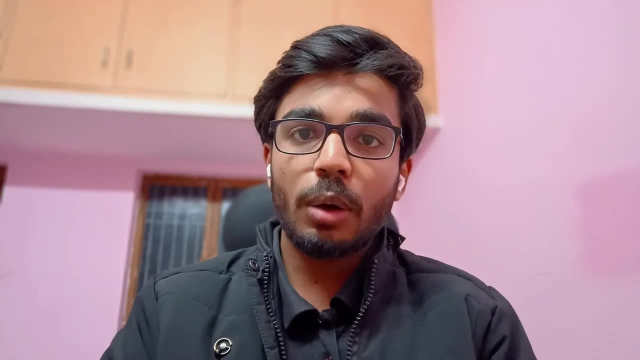 Hey everyone, in this video we will learn what is decorative design pattern. So decorative design pattern are structural design pattern. So what it do is it attach new behavior to the existing object. and how do it? by placing it into a special wrapper object and the behavior 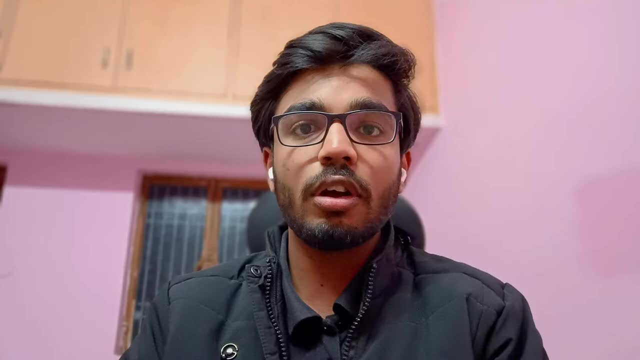 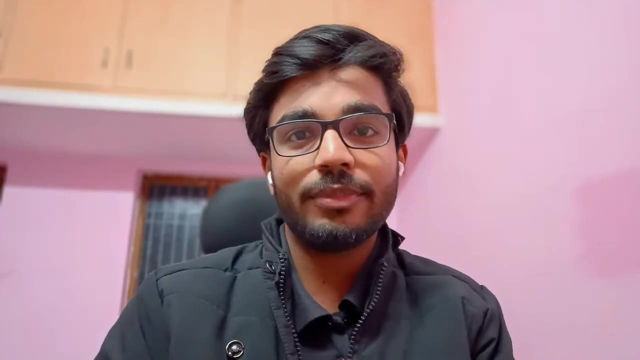 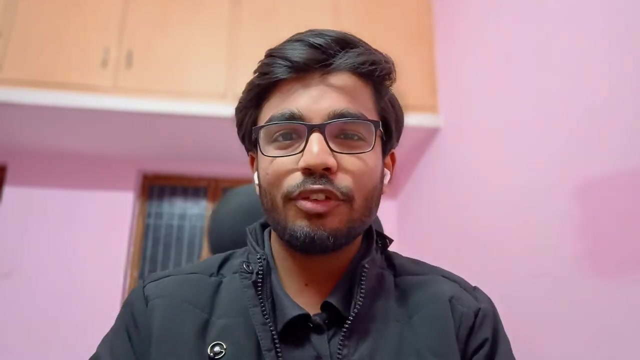 we are talking about to add into our existing object. that behavior will also be containing by these special wrapper object or wrapper objects- and, as you have heard, I am saying wrapper again and again. So these decorative design pattern are also known as wrappers. So I guess it might be little confusing to understand what I am saying, just how we will. 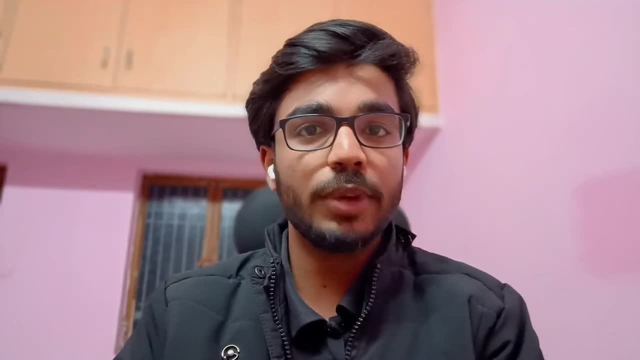 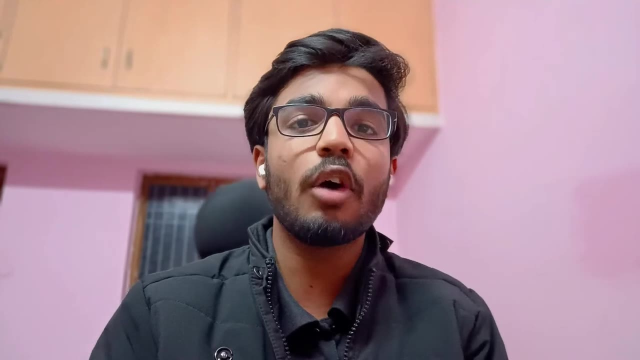 wrap the existing object into a new object and how to attach these new behaviors. So don't worry, you will just understand it by one problem statement, and then we will also write code in Java to understand how it works. So let's understand the problem statement. 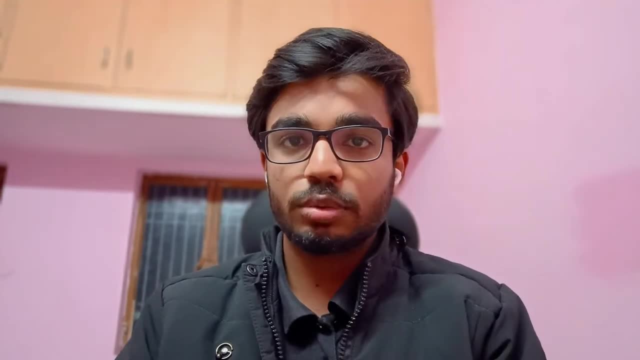 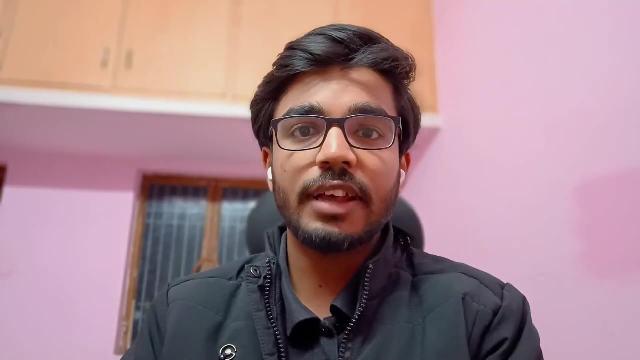 Suppose you are writing one notification library for your customer or like for anybody or your team to use it. So in the initial version of your library you have, let's say, one class which has like notification class and that class has just one method to send notification and it will. 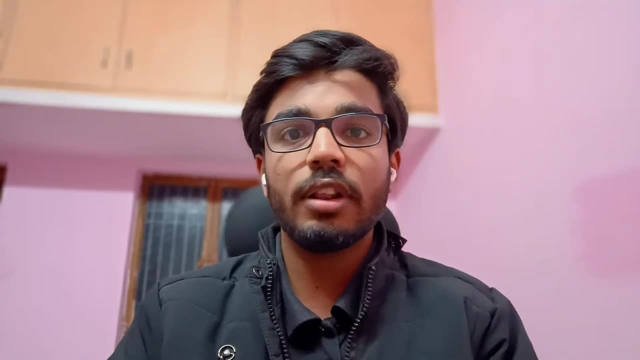 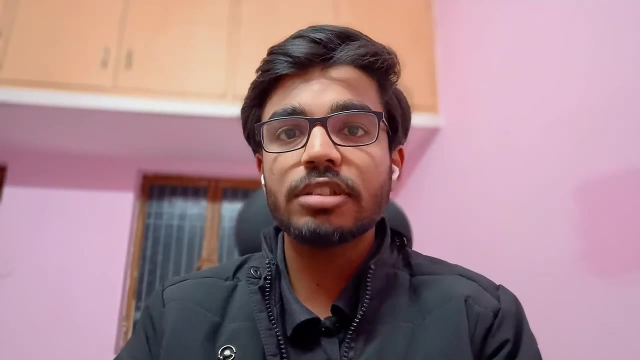 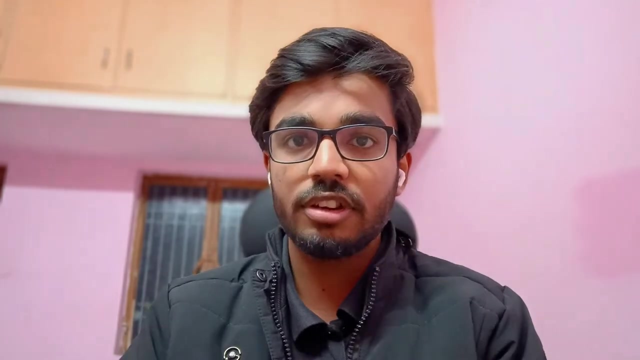 take input as what is the message and list of all the emails to where to send this notification. But in the current scenario it only supports that email notification on emails. but after some time, let's say requirements comes in and you want to support notification or different. 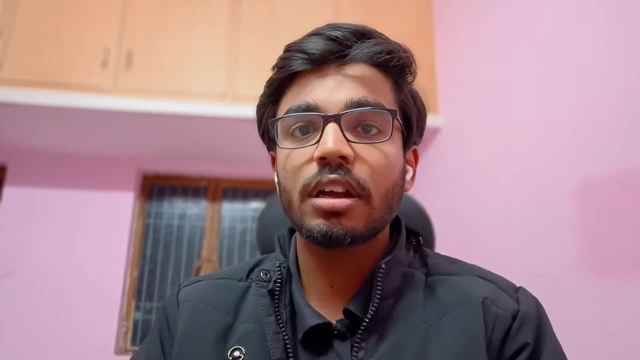 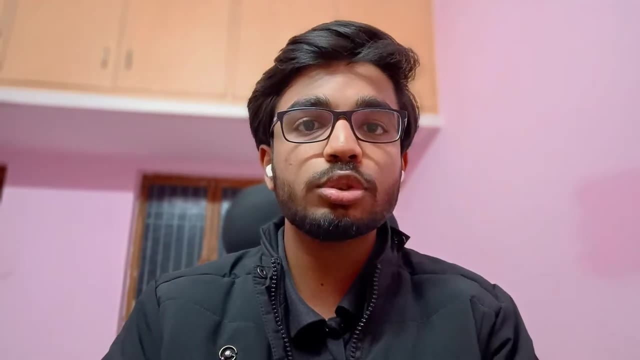 different type of notification on different types of notifications. So in the initial version of your library you have, let's say, one class which has like notification이스ning, and you want to support notification and you want to sign on various different platforms, like on Slack or on phone, SMS, on Facebook or any other channel where 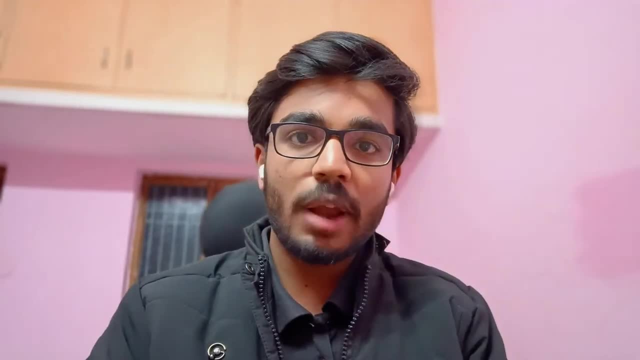 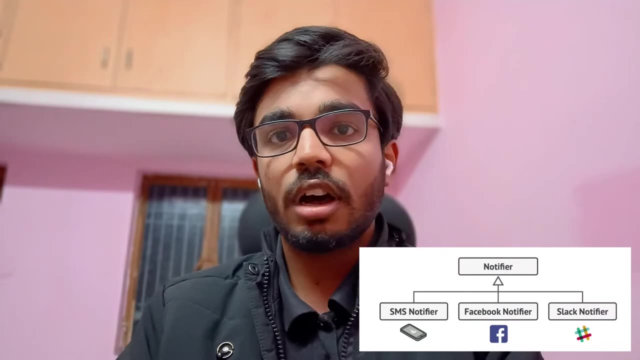 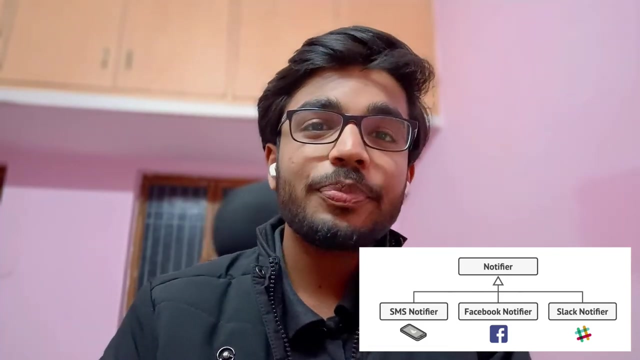 your user wants to get notified, right. So once the little new requirement comes in, it will be any easy to solve that kind of requirement who? what we will do is you just create subclasses with the new, that notification class and extend them. Keep extending it, keep extending it. extending, that is extending it to the new classes. and 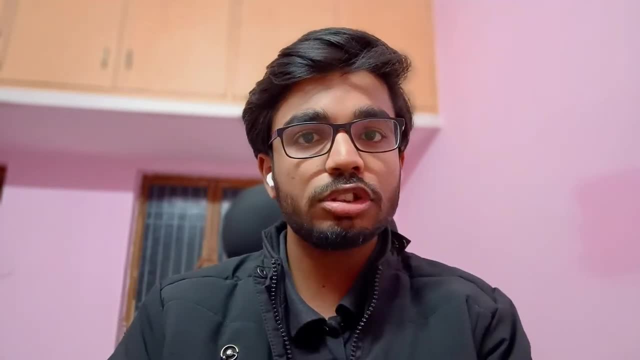 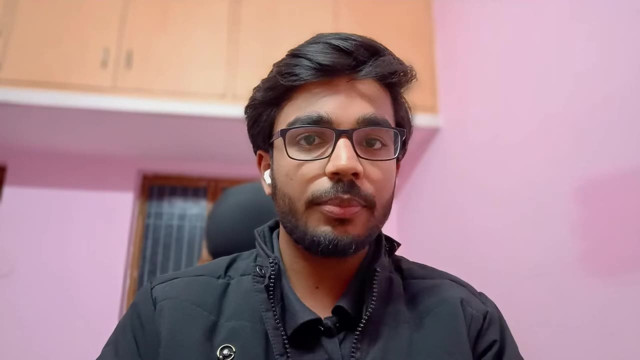 write different, different notification classes and if customer wants to use that notification class and for, let's say, slack, you can use slack notification class or facebook or sms anywhere. but let's say the key point which will give us why we will use the equator design button. 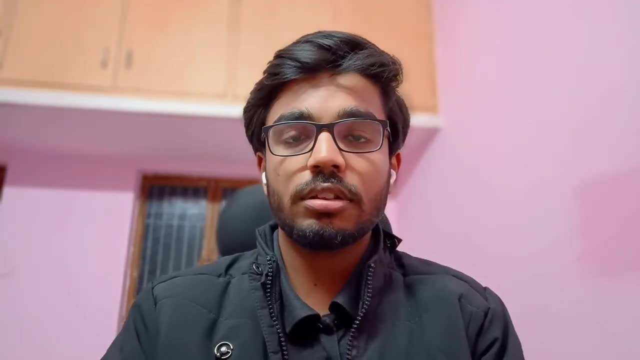 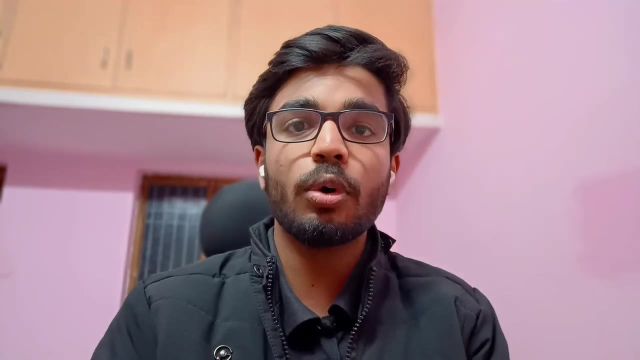 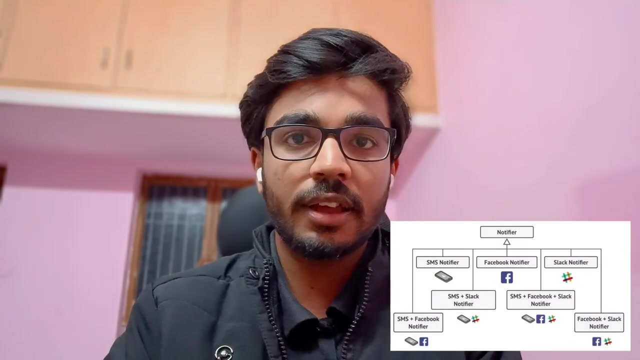 let's say somebody wants notification at all the channels like it is a very crucial issue or something. somebody wants notification at sms, at facebook, at slack and email everywhere. or let's say somebody- sometimes anyone- wants motivation only on slack and sms and other combinations. right, so these combinations will grow as a requirement will grow, so there will. 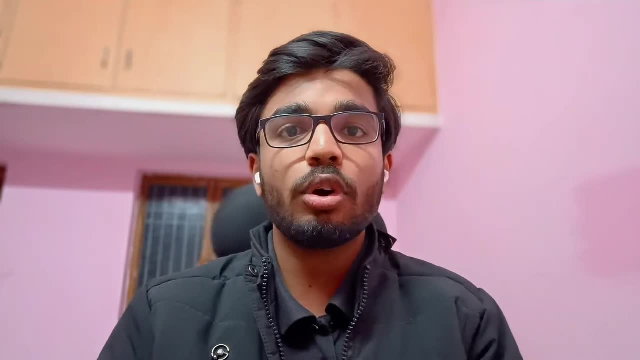 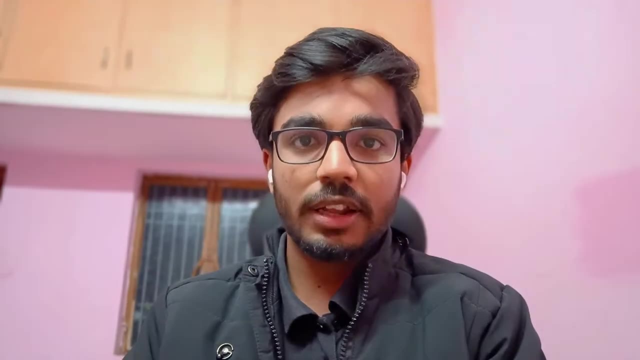 be a lot of code redundancy and also it will, like you know, the code will bloat, because there is a lot of redundancy and we also need to maintain, and not at only the library what we which we are writing, but also at the client side, because he has to create, the client needs to create different. 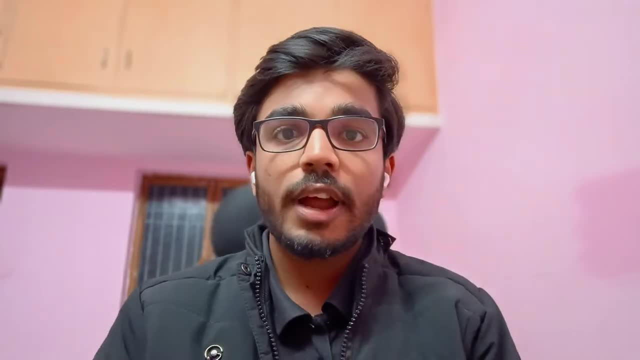 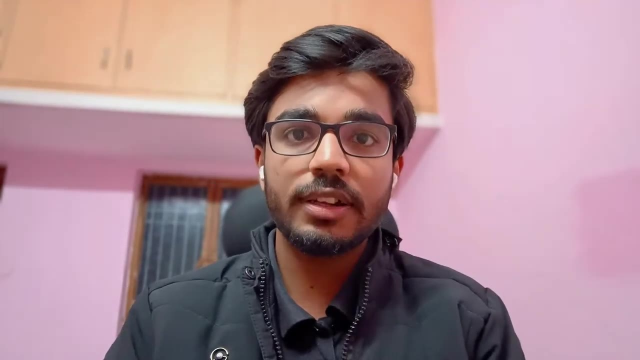 other objects according to the combinations. And to solve such kind of problems we will use Diagorita design pattern. Don't worry, we will just write code and understand how exactly it works and how it will wrap the object, how it will add more functionality. We will see everything. 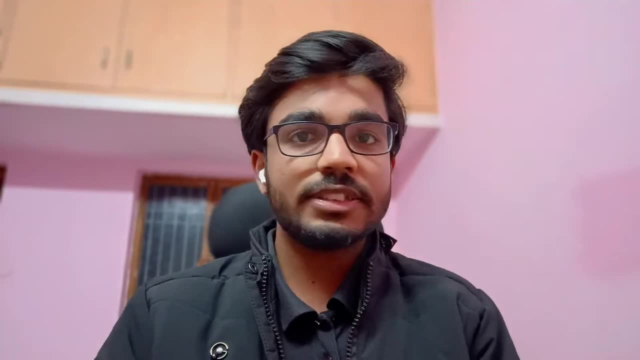 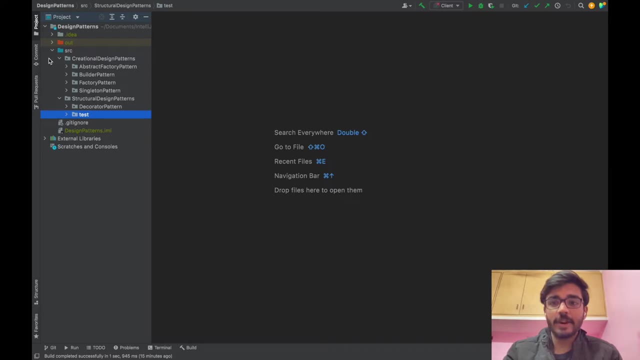 in detail and also write the code. So let us start writing code and then see how it works. Okay, let's write code and see how it works. So far we have covered creation design patterns. You can go and check out those videos also, And all the code is available. 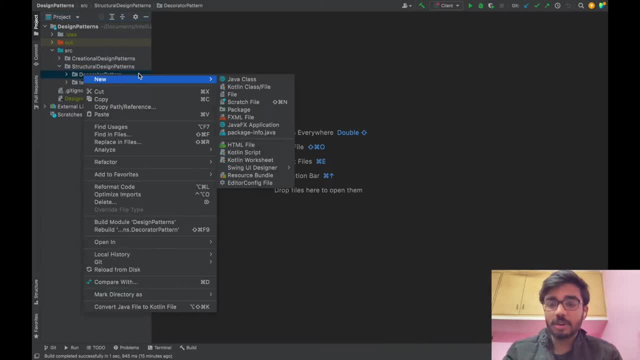 on the GitHub So you can also go and check out. Link is in the description box below. So first we will create our basic notification class which will send notification only to email. So before that we will create one interface which we will call notification. 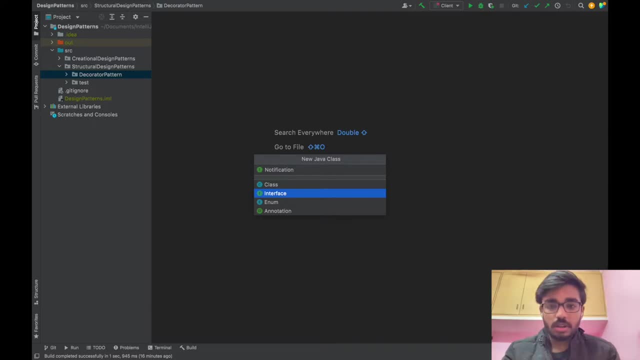 interface, Okay, and this interface, okay. this interface will create one method, one method. So we will create one method, one method, one method. So we will create one method, which is our basic public method to send notification. Yeah, Now we will create. 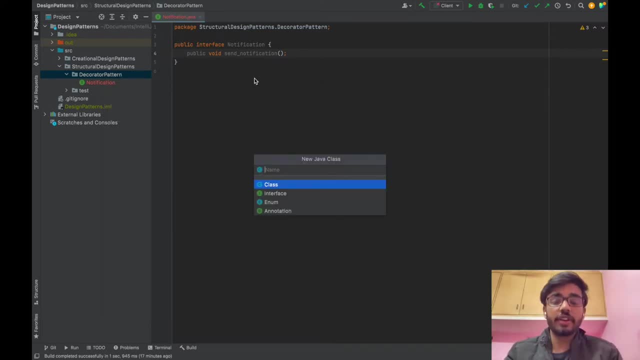 one notify class which will send notification only on email. We will say notify And this notify class will implement this notification interface Notification. So we will just override this method Right, And we will say s out sending email notification Right Now. we will create one. 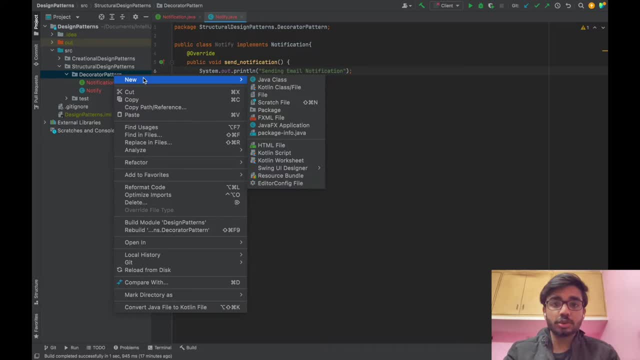 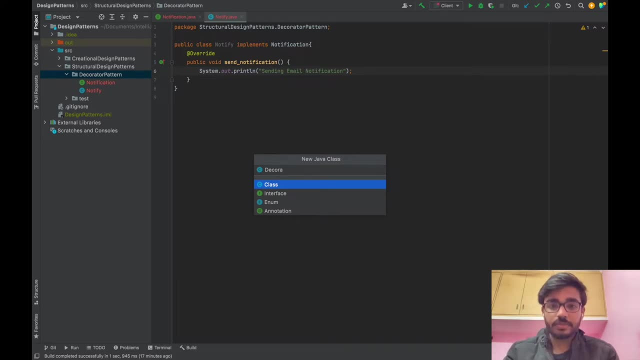 decorator class And this decorator class will help us to create those wrapper objects. You will just see how it works. We will create one decorator Decorator class And this decorator class will also implement our notification interface. It will also implement notification interface And override this existing method which we 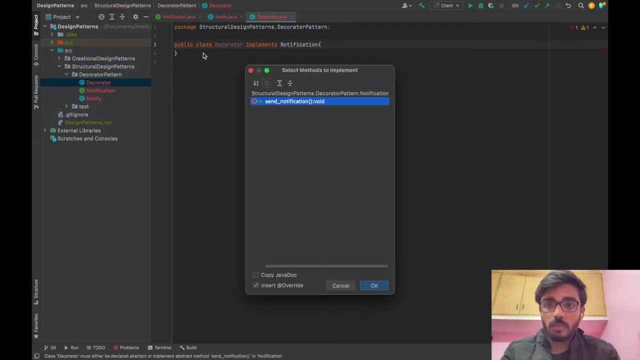 have. Yeah, Okay, But this will create. we will create one constructor here. Let's say, first create the private notification reference And then this we will initialize with the help of constructor of this class. We will say public decorator constructor, which will take one notification argument and initialize. 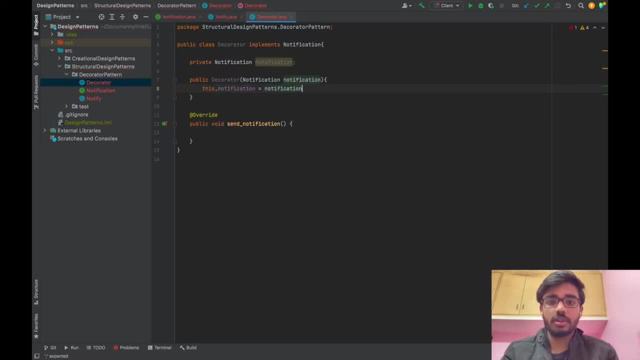 this notification equals to notification Right Now in the same notification. what we will do is we will call the same notification method of this notification, This one. So we will say this dot sign notification Now. just see, now we will create two classes: One, 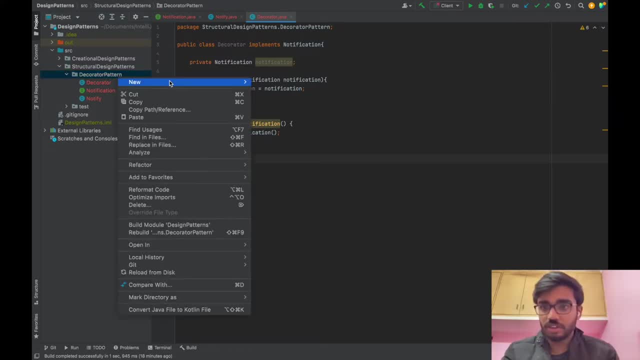 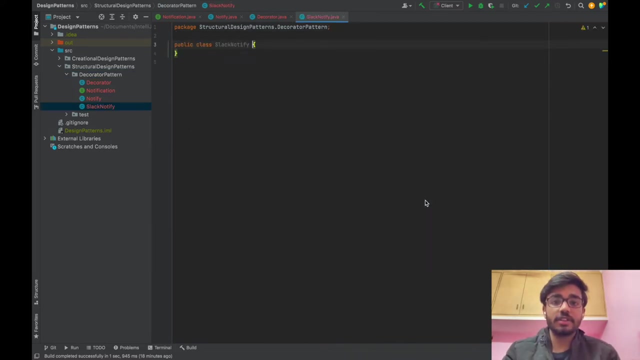 was Slack and one for, let's say, Slack and SMS notification. So first, let's create Slack notification, Slack notifier, We call it Slack notifier. Okay, And this, these classes, these will give us the wrapper objects. Yup, So all these classes will implement. extend this decorator class. You will see. 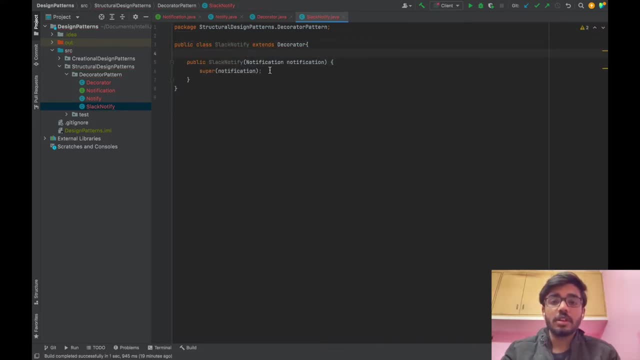 Yeah, so what it does it? it will take the notification and then call the constructor of the super class, which is decorator in this case. Okay, So in this constructor, we will initialize this notification reference with a wrapper. Okay, Soaksha, so I just got a little better with every one. It's a big RiceValue 콘. 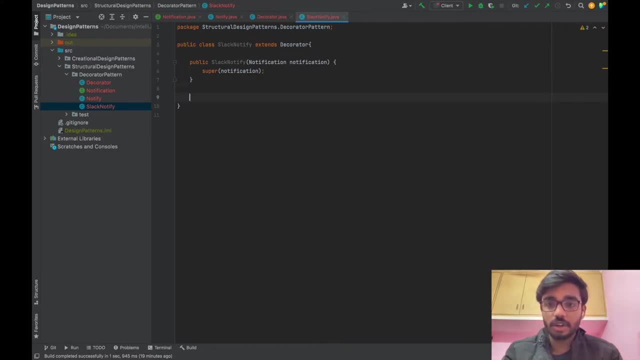 uh, with the object, we will pass here and we will just see how it works. and we will and we will also overwrite the method, that's this send notification method here and this. this is how we will achieve that, adding additional feature. we will just see how it works. okay, so first what we 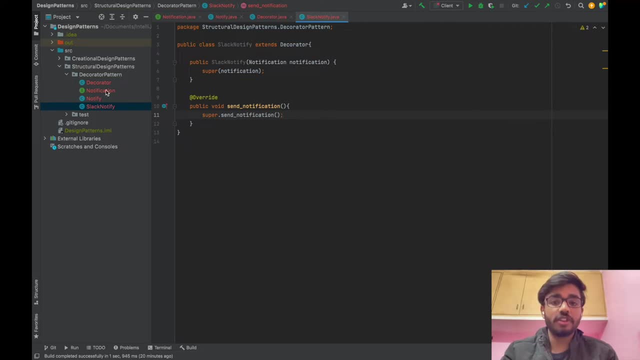 will do is: okay, call the send notification of the super. like already existing features. now you have already existing features. now i will add my features, which i want to add to that. like once, when we, once we wrap the object into ourselves, we can just the features of the object and also. 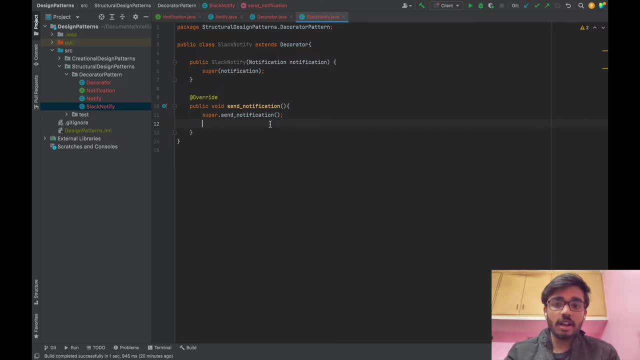 add some additional object and additional features, and here we will add the additional feature. let's say, now we will say s out and we will call it this: sorry, sending slack notification. let's remove this from here and remove this from here. okay, now we will create one more class for sms notification which is exactly like this: enough, no, it is called. 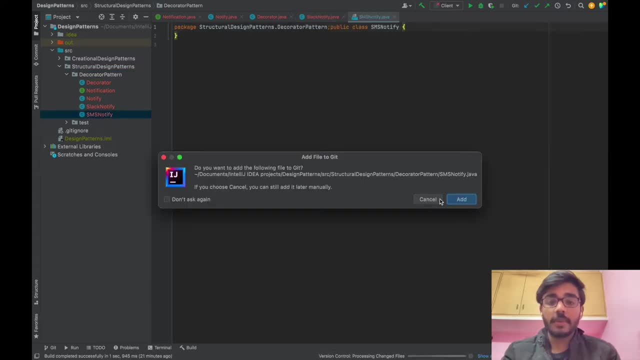 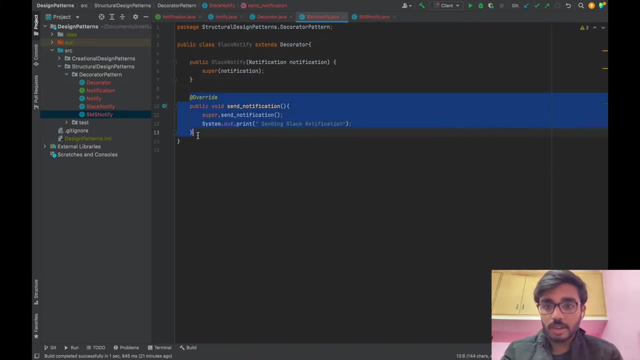 sms which is exactly like this: enough. no, it is called sms which is exactly like this: enough. no, it is called sms s notify, and we will say: extend, not decorator class. create the constructor with the super, and we will say: we'll check. copy this from here, actually, and overwrite the send notification. 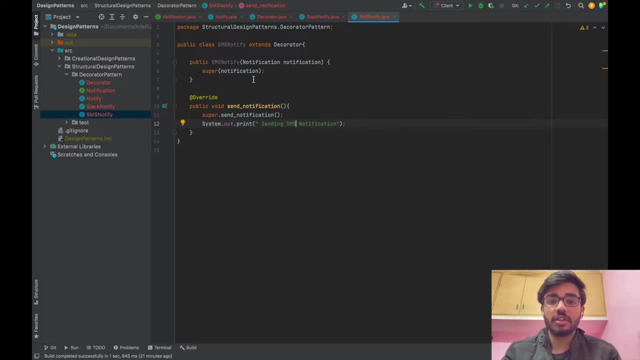 method, and here it is sms notification, right? so this is how it works. now let's create one client class, and then it will be more clear that how these things are working. let's add this public static void main. okay, so first you will create the basic object of our notify class, which 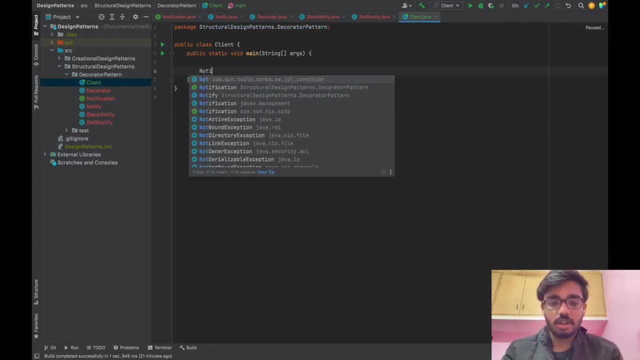 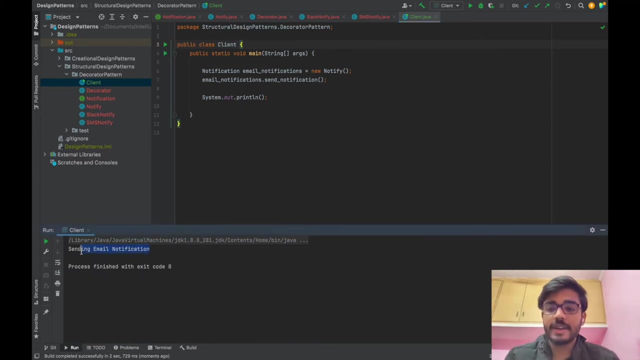 will send notification only to email. so we will say: notify email notifications. oh, even we will call it notifications, because it implements the notification interface, new notify right. and here we will say this: dot sorry, email notification, dot send notification. yeah, so if i run this class i am getting only email notification. but now let's say i want email as well as. 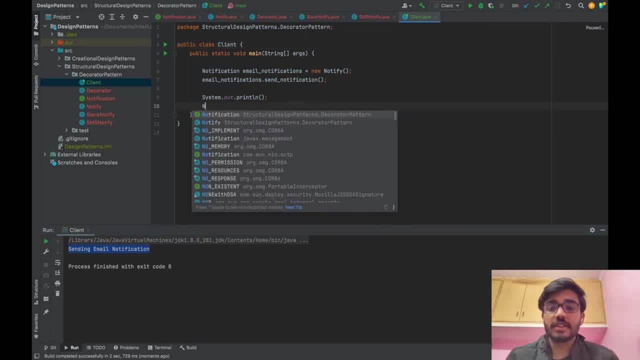 slack notifications. so what i will do? i will just create notification, slack notification notifications. slack and email notification equals to slack notification. now, here it will give me the feature of slack notifications, but in this i will also wrap the email notifications. so see how it works this. so this is my current object and this is the new object i am creating and this is my wrapper. 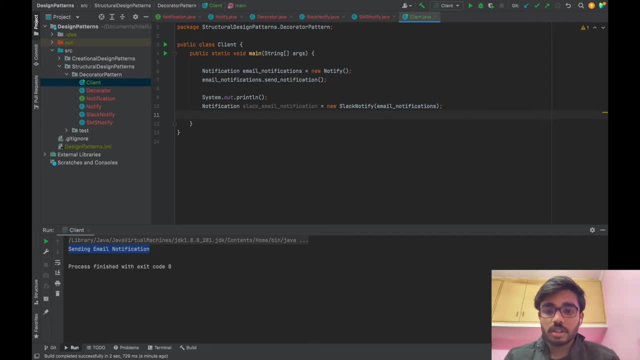 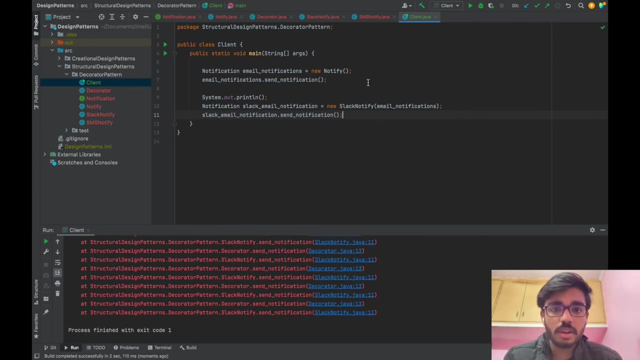 object in this. i am wrapping my email notifications. so now i'm say slack email notification, that's dot send notification. and if i run this now, okay, we got some error, okay, okay. okay, let's solve this super notification. i am saying what i am saying, where is the client? yeah, slack notification, where i am saying email. 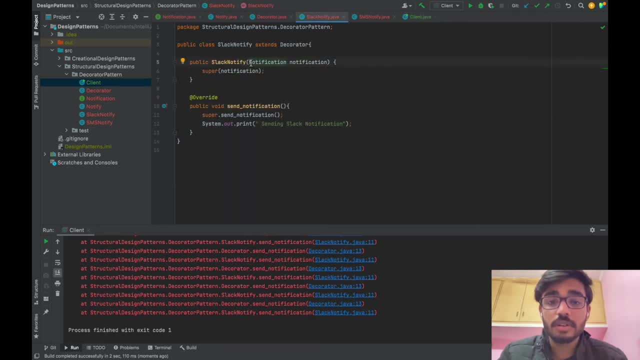 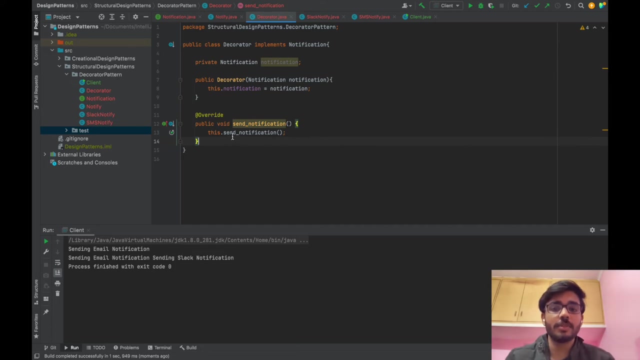 notification on the slash notification. email notification will go in the super, which is actually a decorator. yeah, okay, so i found the error. this is previously we had this: this dot sign notification. okay, and now, if you cl, check this out, but it is incorrect because we need this. what is this? is a notification when we said this dot. 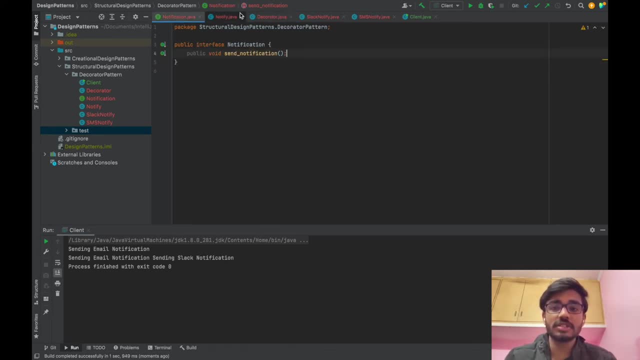 notification. this dot send notification. it will just go here, but we so it will call a notification of all the classes which is implementing this notification interface. but we need only to call the send notification method of this particular notification. like with who it is different. like we will say, this notification, let's say, get initialized with the slack notification for now, 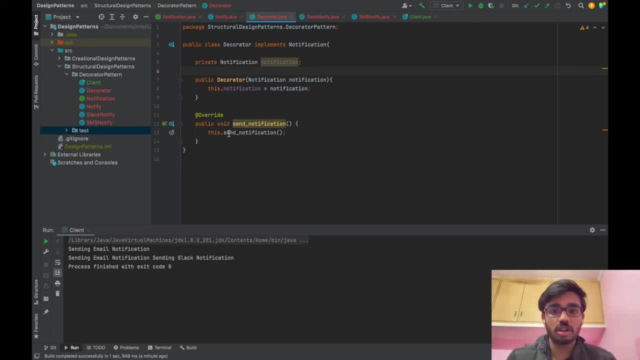 so we only want to call the no send notification of the slack, not all. so we will say this: dot notification, dot send notification, or it was also giving us the warning which we ignored now, but and if we run it now, this will send us sending email notification for this and sending. 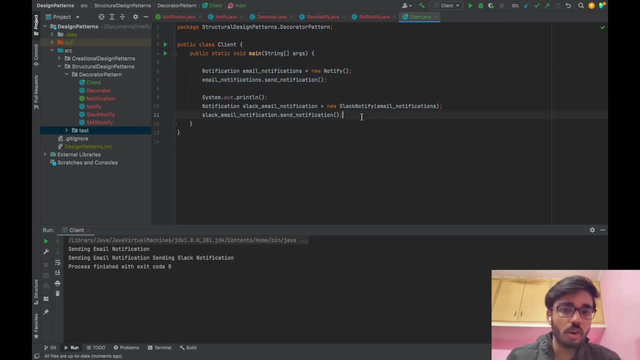 email notification and sending slack notification, which we want. now let's say same thing we will do for SMS. I want slack email. or even say I want SMS and email notifications. so I will just say SMS notify. and now I am wrapping my email notification into SMS notifications. and if I run, 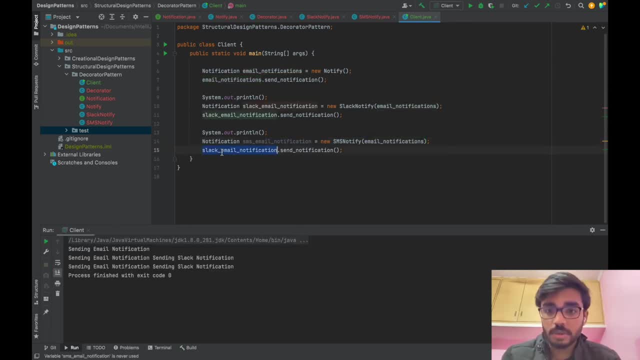 it now. okay, this should also be updated so that it will be same. this is sending email notification for this, sending email notification for this, sending email notification for this, sending email and slack for this one and sending email and SMS for this one. now, let's, I want everything which. 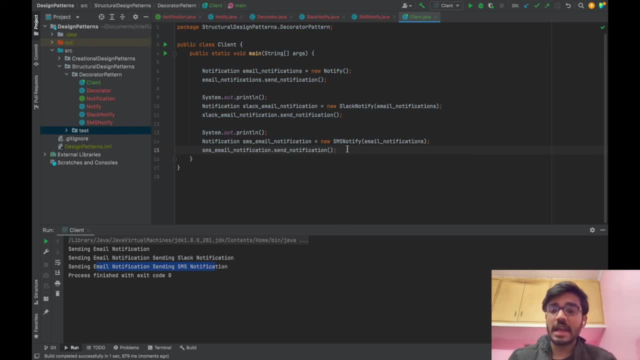 is the important use case we discussed. I want email, I want slack, I want SMS. so what we will do is just the same thing. actually, we will say notification all equals to new. let's say I will say slack, not SMS, notification. in the SMS I will wrap my slack notification. 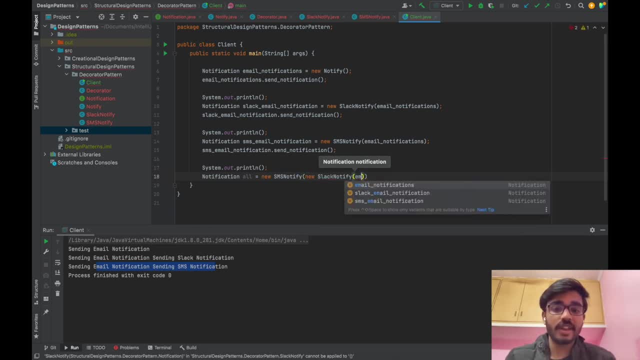 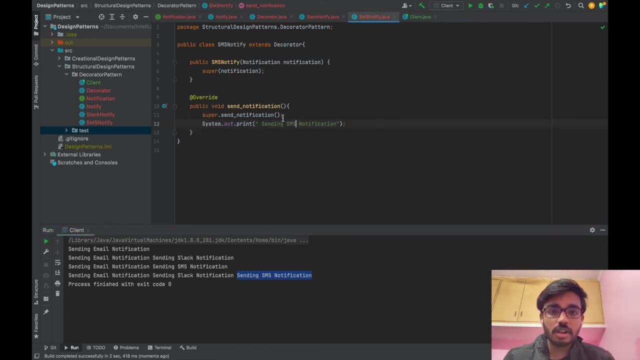 in the Slack, I will wrap my email notification and now I will say all dot send notifications. so see, we got email notification, we got send slack notification as well as we got SMS notification. so this is how it works because, like say here, we call the super notification tool. it give us the features.